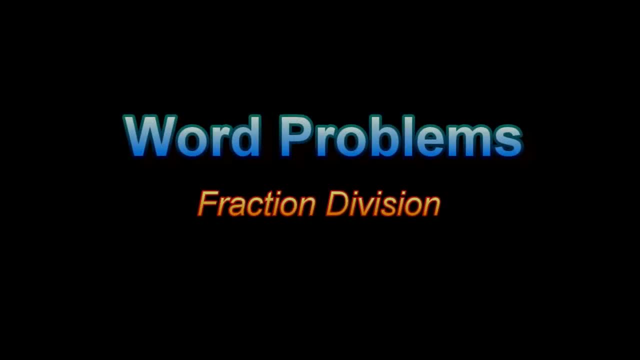 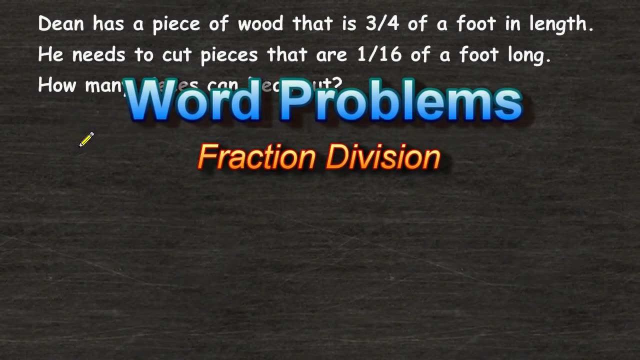 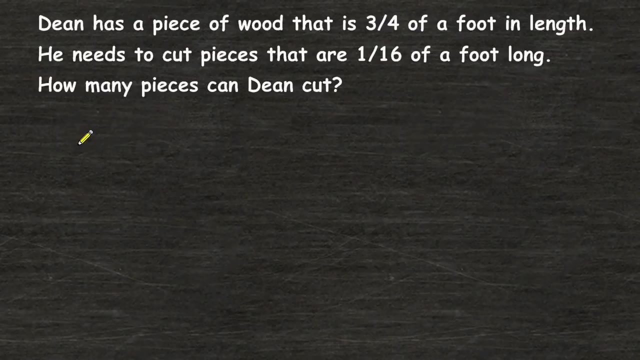 In this problem. it says that Dean has a piece of wood that is three-quarters of a foot in length. He needs to cut pieces that are one-sixteenth of a foot long. How many pieces can Dean cut? After reading this story problem, we should recognize that we can use division to solve. 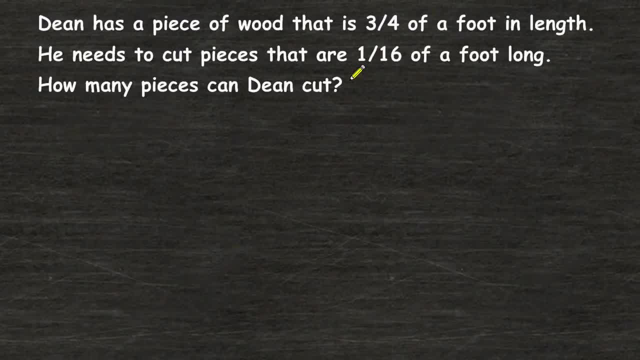 Basically, we are trying to figure out how many pieces of wood the size of one-sixteenth of a foot can be divided into a piece of wood that is three-fourths of a foot in length. So one thing we can do is take three-fourths and divide that by one-sixteenth. Be cautious. 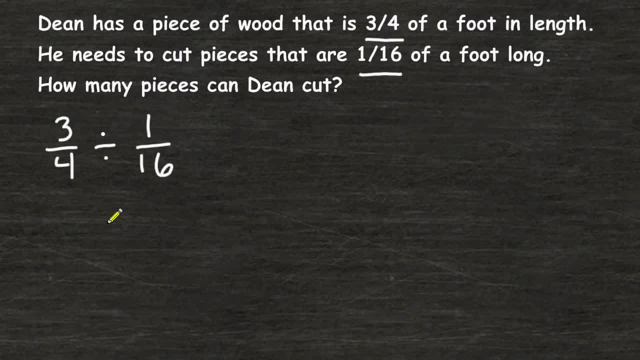 when setting up a division problem, because the fraction you write first and the fraction you write second is very important. If you were to put the fractions in the wrong order, you would come up with the wrong answer. Just remember that the amount that you are starting with, that is to be divided up or chopped up, must be written. 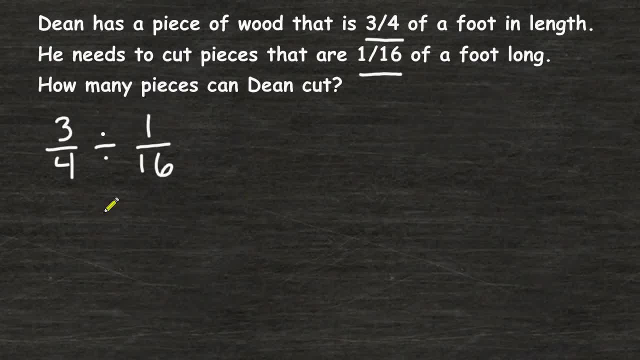 first and the other fraction go second. After setting up your problem, rewrite the first fraction and multiply it by the reciprocal of the second fraction. So we are going to multiply three-fourths by sixty-eight. After that, the mixture is equal to sixty-size những-ti-sixteen over one. 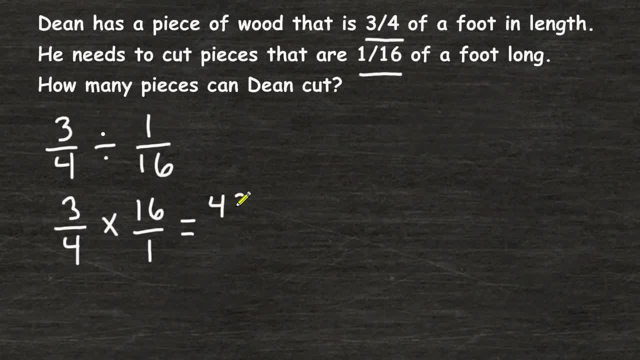 Now, the first is going to have a product of four. The next thing we can do is multiply the numerators together. Three times sixteen is forty-eight and the denominators have a product of four. Because we have an improper fraction, we are going to divide the numerator by the denominator. 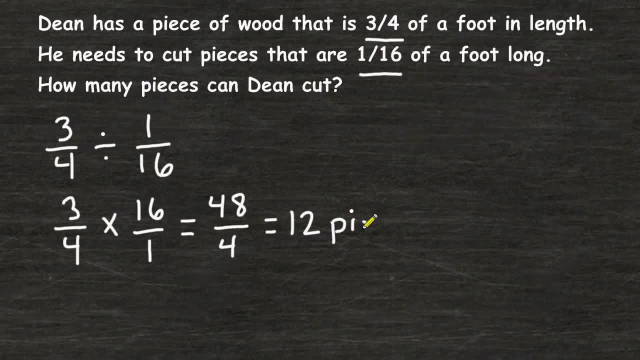 and forty-eight divided by four is exactly twelve. So if we were to cut a piece of wood, 12 pieces that were the size of 1 16th of a foot long. Another strategy that we can use to solve this problem is by drawing a diagram. 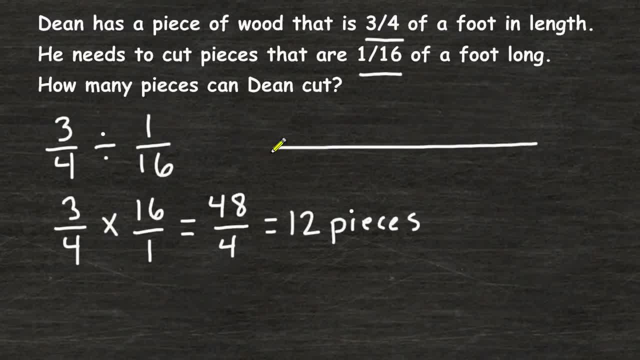 So I'm going to start by drawing a line that represents the length of the piece of wood, and I'm going to start by marking the beginning of that piece of wood as zero. We're going to say that this right here is 1 foot, halfway of course is 1 half of a foot. 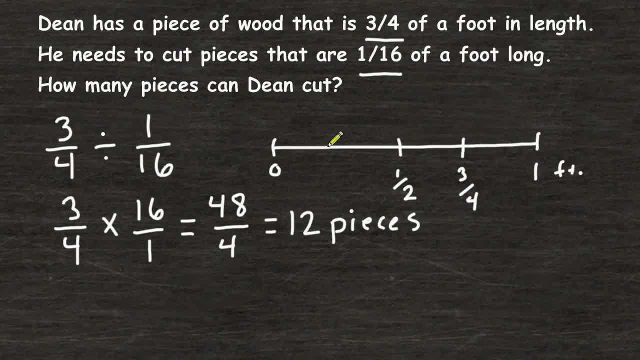 this would be 3 quarters of a foot, which is actually the length of the original piece of wood, and this mark right here is 1 fourth of a foot. Now it says that Dean wants to cut his wood into pieces that are 1 16th of a foot. so 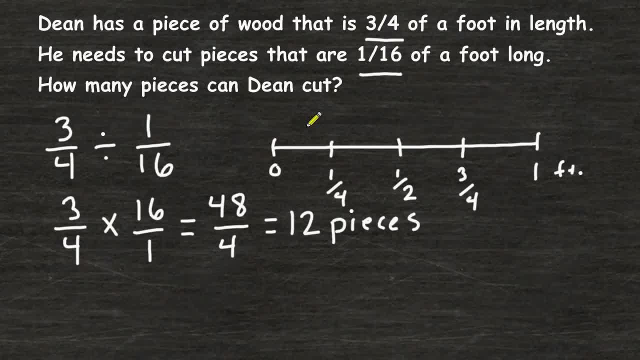 now I'm going to divide this entire foot into 16 pieces, So this quarter has to be broken into 4 sections, this quarter into 4 sections, this quarter into 4 sections and this quarter into 4 sections. Now all I simply have to do is see how many times I can fit 1 16th into 3 fourths. 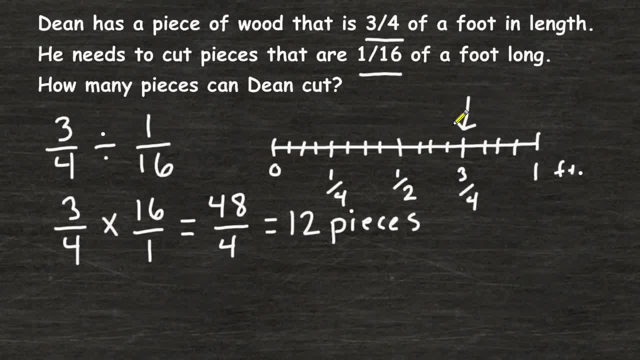 So I must stop when I hit this mark right here, because that's how long the piece of wood is, And from this point to this point is exactly 1 16th. So that would be 1 piece of wood, 2 pieces of wood, 3, 4,, 5,, 6,, 7,, 8,, 9,, 10,, 11, and 12.. 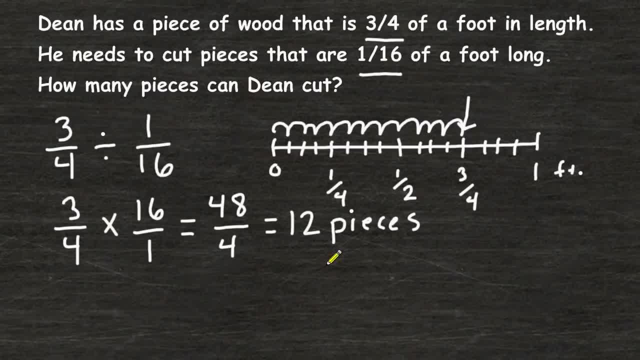 So we can see that 12 pieces of wood the size of 1 16th of a foot would fit exactly into a piece of wood that is 3 quarters of a foot in length. Now I'm going to start by drawing a line that represents the length of the original. 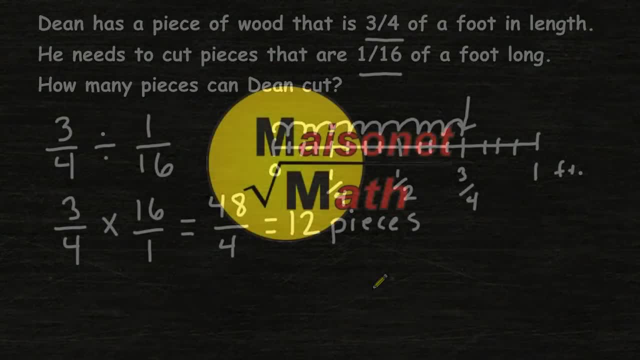 piece of wood. Now I'm going to start by drawing a line that represents the length of the original piece of wood. that represents the length of the original piece of wood. that represents the length of the original piece of wood. that represents the length of the original piece. 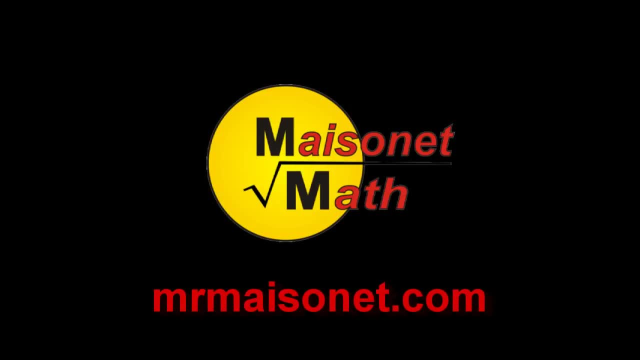 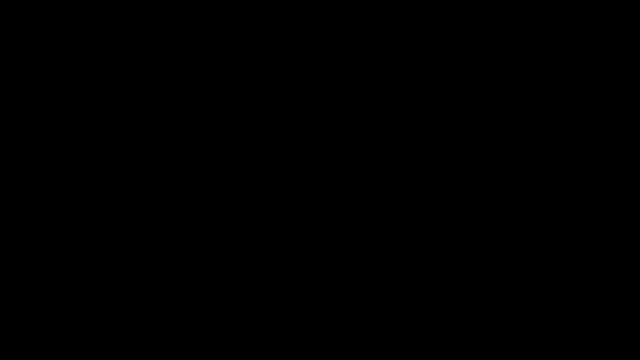 of the original piece of wood. that represents the length of the original piece of wood that represents. Thanks for watching.